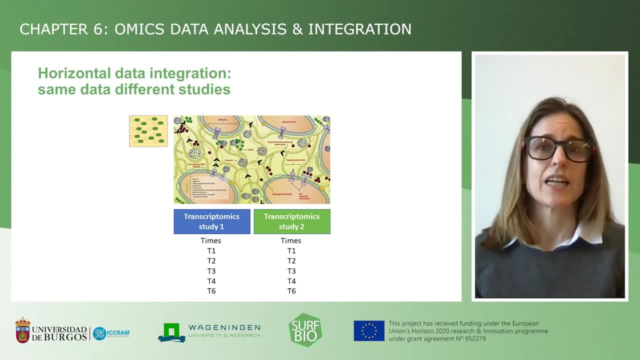 of your biofilm And another lab has collected data on the same sample type that could be added to your analysis. Or you added some extra transcriptomics experiment on the same type of sample but different conditions. In this case, you have the same type of variables, namely the active genes that are measured. 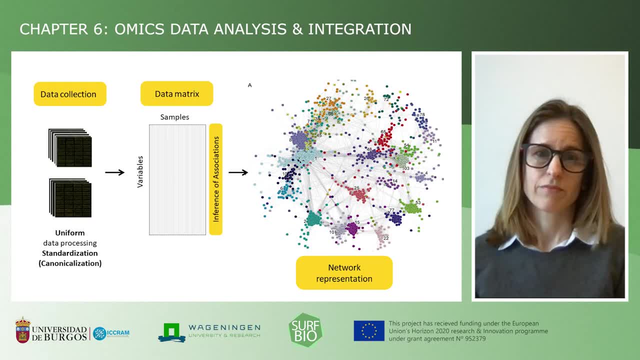 yet coming from different studies. So what is the goal of data integration? For such a case, there is a general workflow to find associations and visualize them in a network. We start by making the data uniform, For example by processing them in the same way, so that you can put all variables and 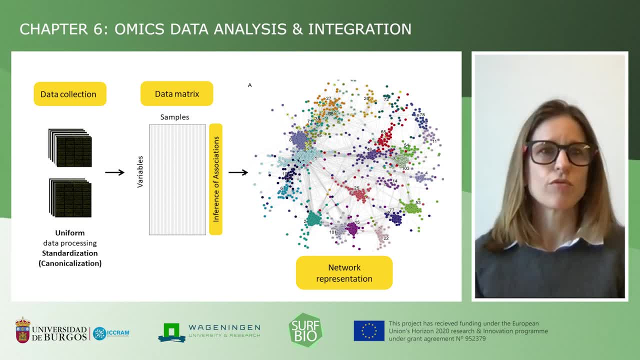 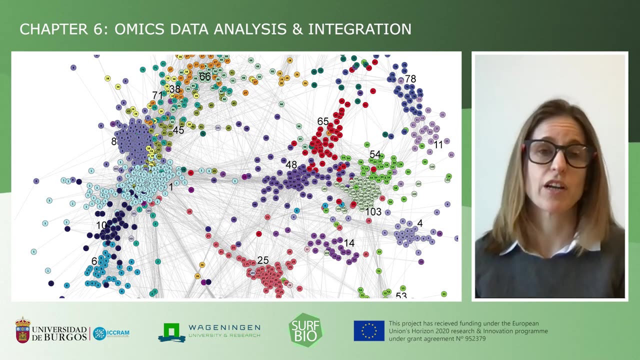 conditions together. We then look for associations among the active genes in this big matrix and build this association via a network representation. A network is a graph of concepts and relations. Nodes, the dot in the figure, represent variables and edges, the connection between the dots. 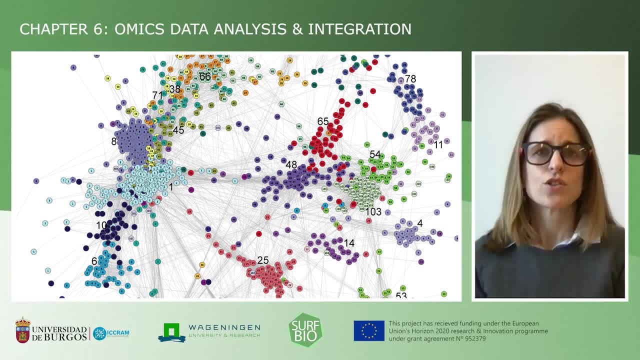 the significant association. So you can already appreciate by zooming in in the previous network that this group, number 25, and colored in red are genes that are shared. So you can see that we are sharing some association or characteristics. 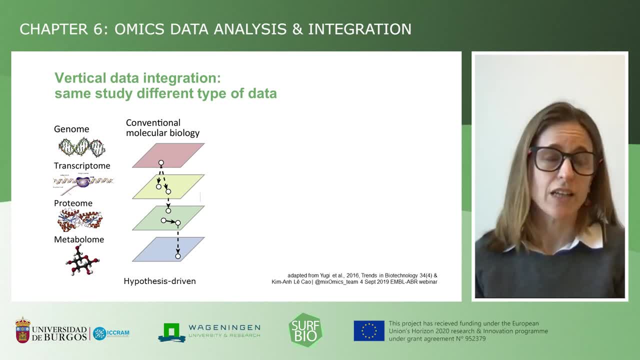 Now let's move on to vertical integration. when we want to join data from different data type collected on the same samples, Why should you integrate data in case of different data type? We can actually study these different levels that bring us from genotype to phenotype using 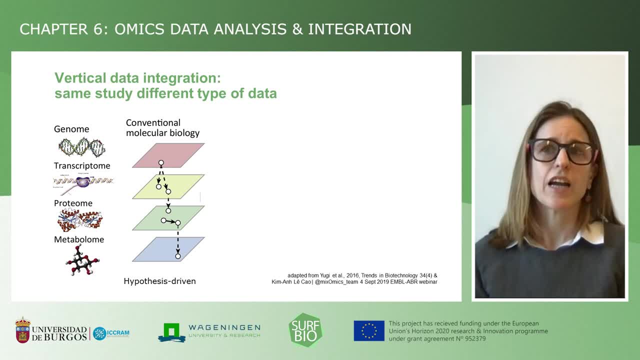 conventional molecular biology tools, Following in such a way a hypothesis-driven approach. In this example, you would study a gene, identify maybe a few targets for transcriptional changes connected to the expression of this gene, then move to the protein level and focus on. 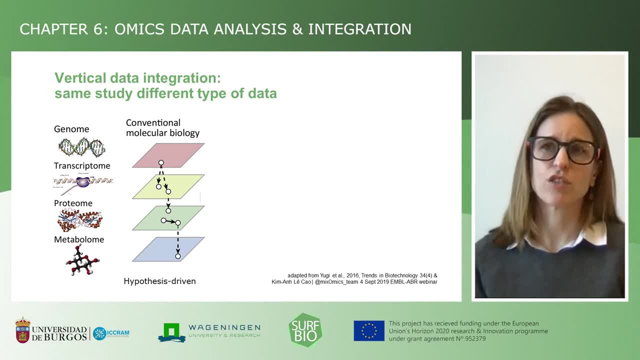 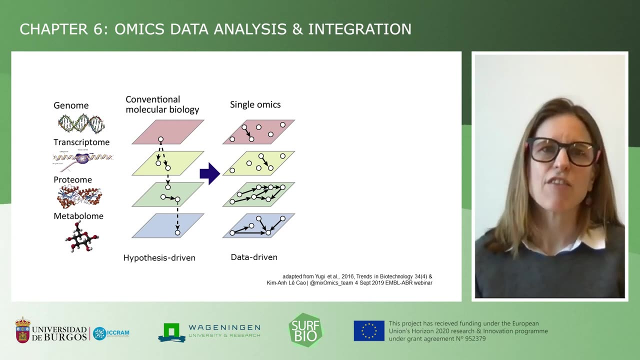 studying its interaction or activity in the case of an enzyme, And finally, look at the molecule transformed or produced by the enzyme and influencing metabolism. With the development of the AMICS technology, we can definitely expand our knowledge on each level, and so we can generate discoveries driven by data. 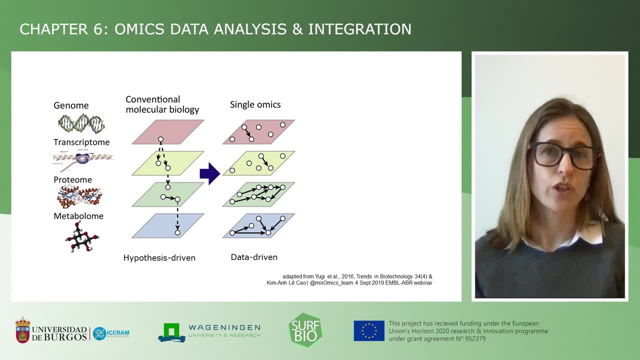 In such a case you would test a general condition or change from the wild-type condition and start from the changes observed to deduce an hypothesis explaining those differences and move to test data. In this way we can really see what the MESA and other underlying concepts of the AMICS. 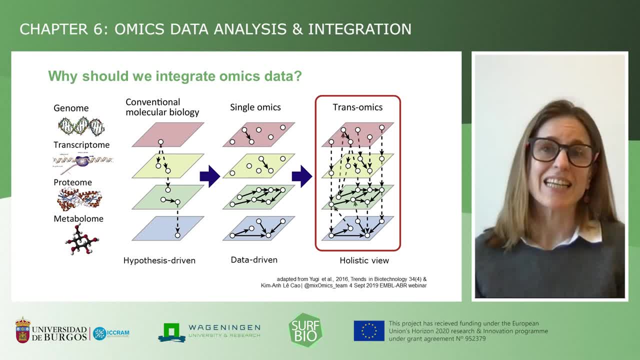 uses to interpret these data theories and how that hypothesis's background can change in the following-up experiments. Yet nowadays we can integrate the different AMICS levels to reach a more holistic understanding of the system. These allow us to get an insight into the relationship between the AMICS levels and 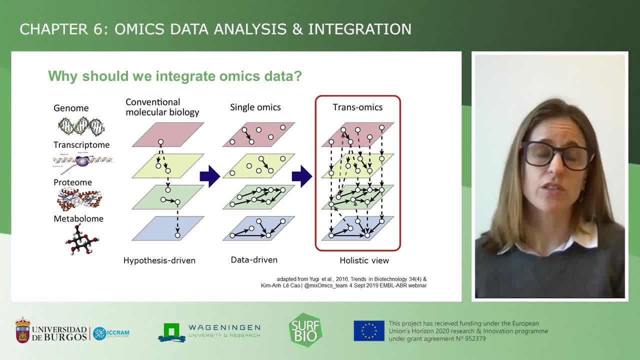 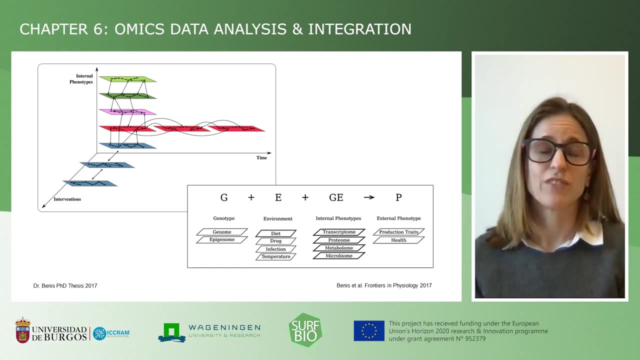 molecular mechanisms describing the condition studies, Predictive analytical models that report a signature for the condition that can be used for future estimation on a known sample of the same type. So, as you can appreciate, the final picture of the data available nowadays is more complex. 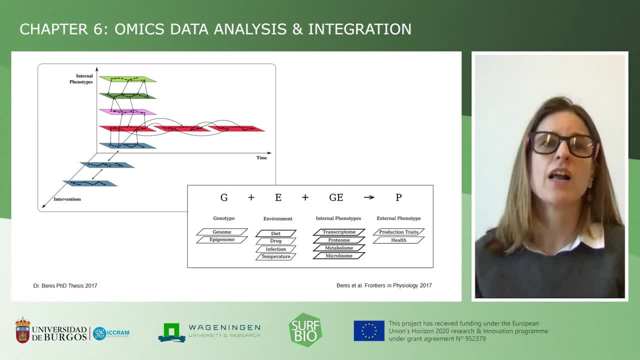 We can have different intervention on different phenotypes, collecting different type of variables, measurements, and all of this in different time. Our aim is then to link the genotype and the environment to the observed phenotype in terms of production traits or implication for health. 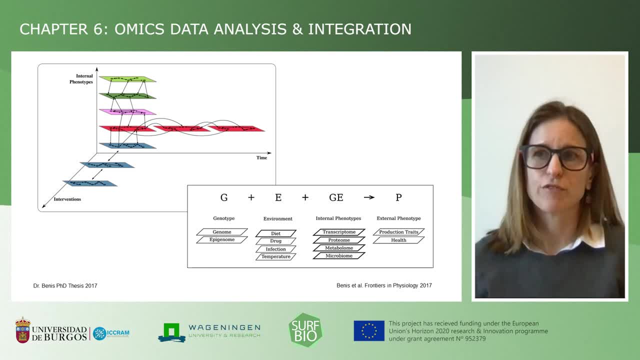 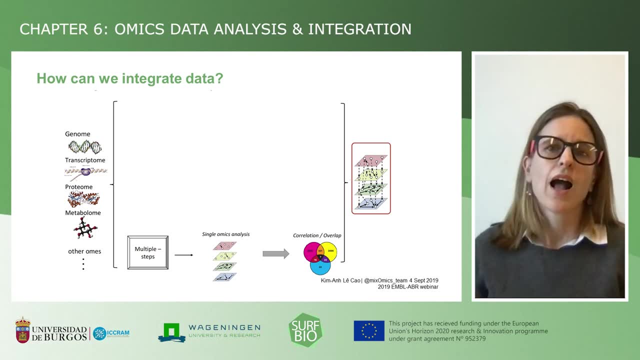 And we do this through the measurement of the different internal variables, so the different omics. Now how can we integrate the data? So we can do that by individual levels, combining individual levels, and look afterwards at correlations and overlaps among the different variables. 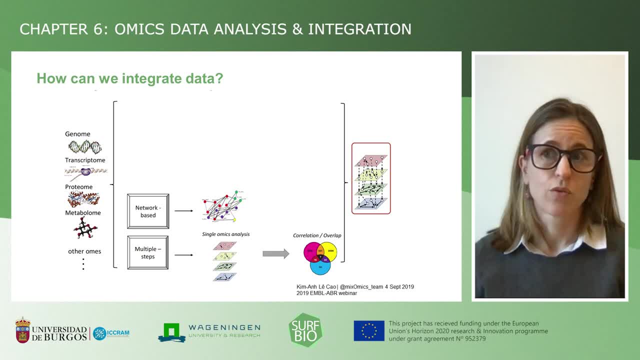 We can also use the data from the data set. We can also use the data from the data set. We can also use network approaches where nodes, in this case, represent different types of variables, so proteins, metabolites, genes. You can use Bayesian statistic approaches to measure the amount of information a data set provides to parameter estimate. 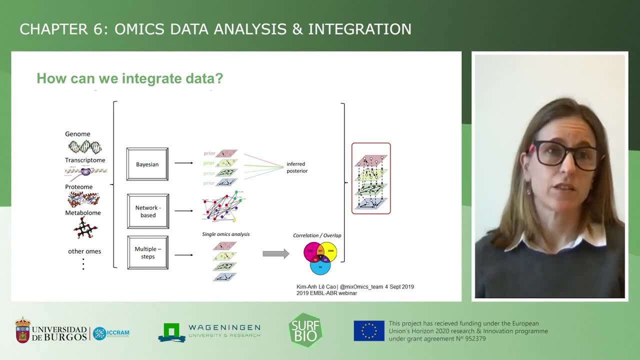